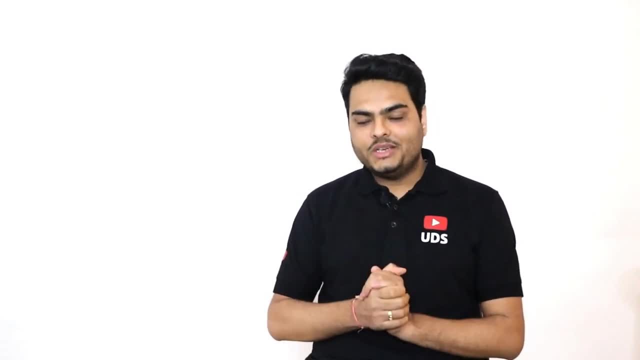 There are some topics which, when you search on internet, you are bombarded with jargons and then you are lost in between jargons. Principal component analysis is one such topic. And why do you come to Unfold Data Science guys? You come to understand things, jargon free. 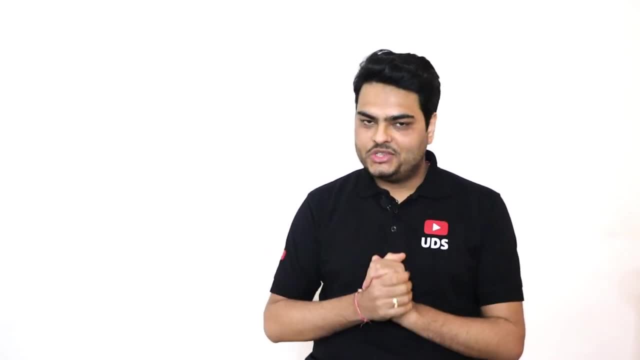 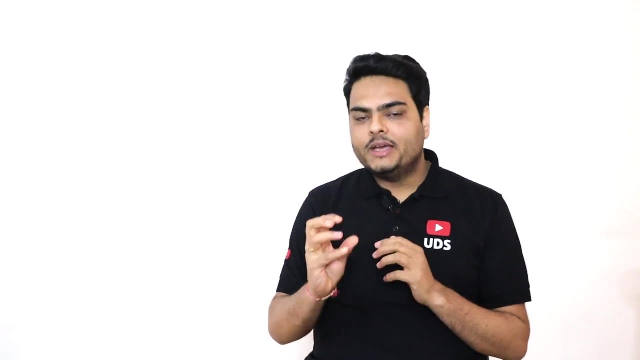 Welcome to Unfold Data Science. My name is Aman and I am a data scientist. What I am going to do in this video is I am going to explain different pieces of a puzzle known as principal component analysis, And in the end, I will combine all these pieces. 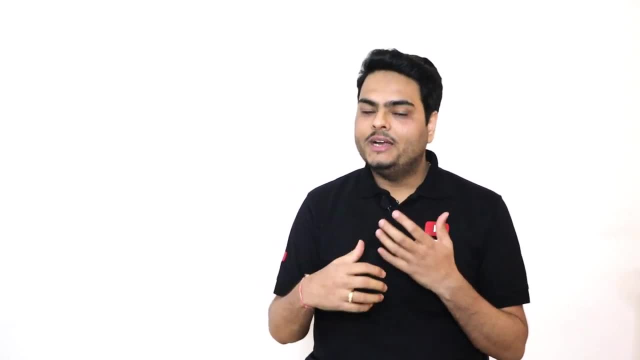 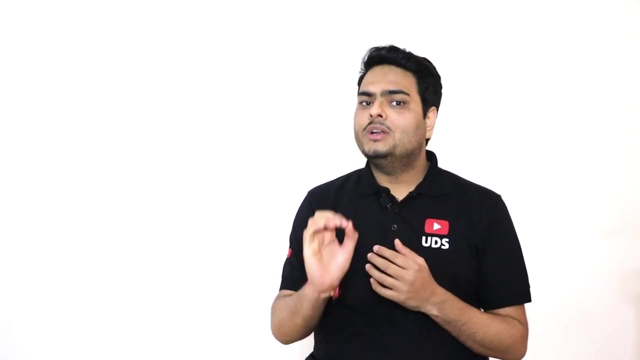 and tell you what is PCA and how it works and what is the internal mathematics, And I will also show you in Python how it works, So that you understand this complete concept as a package. What I expect from you? Only one thing, guys: patience. You already 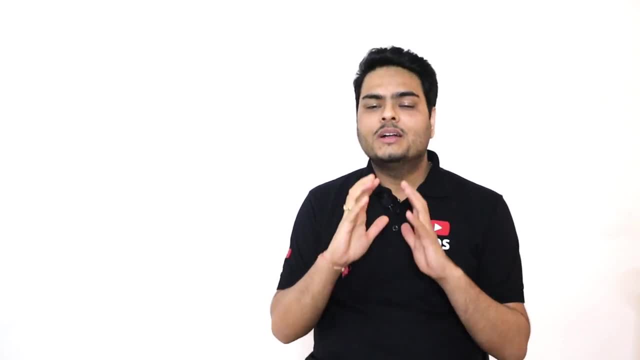 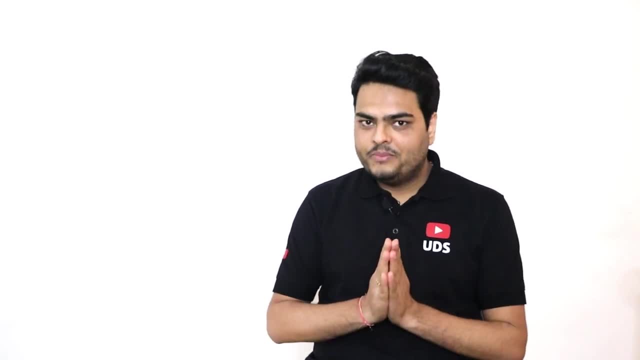 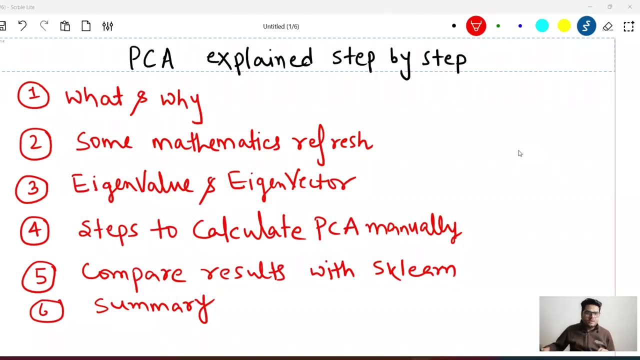 end this puzzle will be very, very easy to understand, so let me take you to the whiteboard and try to explain different pieces of this puzzle. okay, I have written here. I am going to explain many concepts in this video, because if I skip any of these then it will be difficult for you to understand PCA, okay. 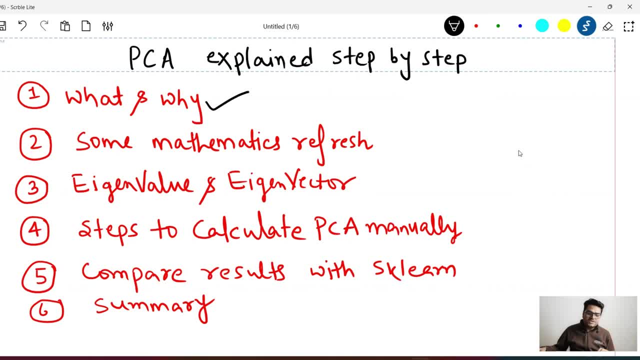 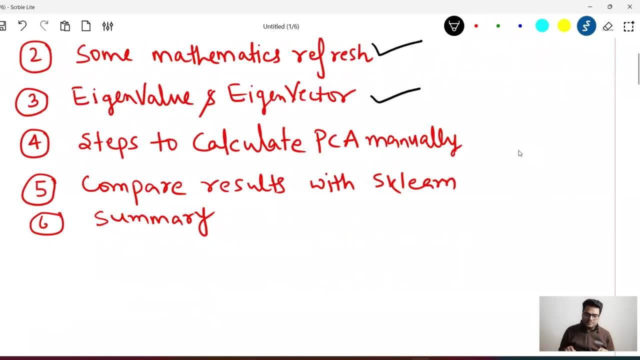 so first we will understand what and why of PCA and then we will go and do some mathematical reflux, because it is necessary for you to understand PCA. then I will give you some examples of eigenvalues and eigenvectors, which is very important to understand from PCA point of view. most important guys, we 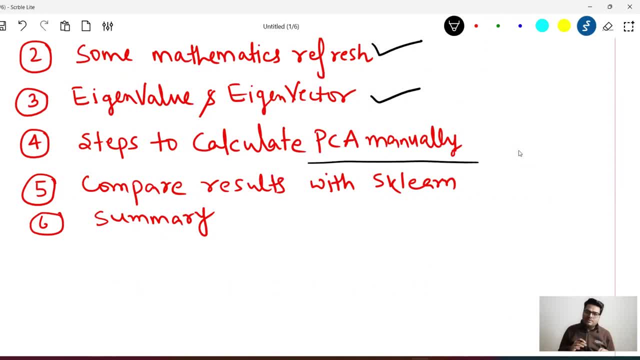 will do manual calculation of PCA, which means we will not use sklearns PCA. we will do the manual calculation and then see how it is coming out and we will compare with sklearn PCA and then in the end I am going to tell you summary of our learnings and 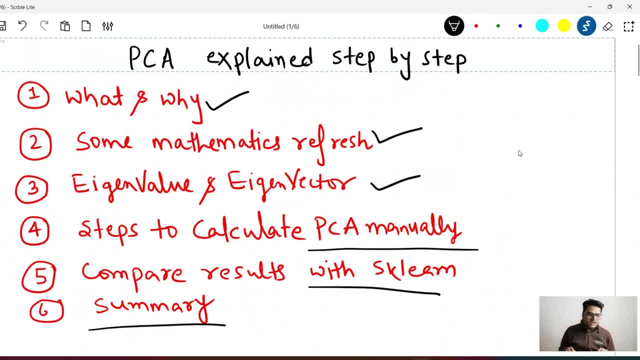 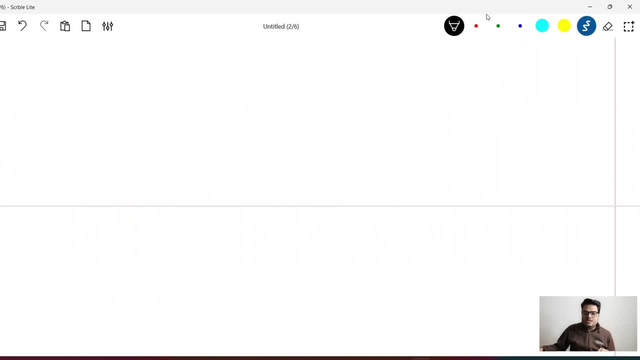 what are the limitations of PCA? okay, so let's start, guys. lot of things to cover without any further delay: what and why of PCA, right? so what is PCA, guys? if somebody asks you, PCA is nothing but a feature reduction technique. feature reduction technique. why feature reduction technique is needed in a data? 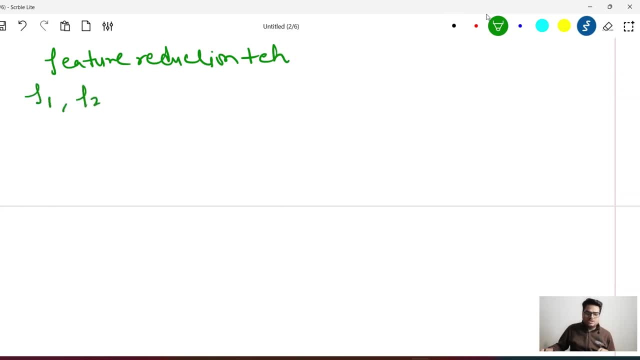 set. there can be many features, for example feature 1, feature 2, up to feature red. all these features are not equally important. you know from your data science experience, right? so feature 2 may have same information, more or less, which feature 5 is having in that case. I don't want to overload my model with 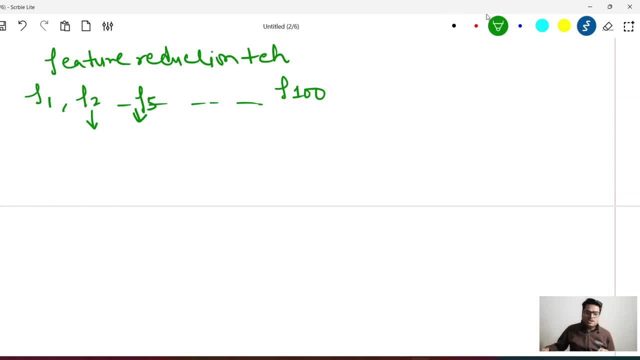 redundant information. hence I want a solution to reduce the feature at the same time. at the same time, I do not want to extract the meaningful information out from the data. so to solve this issue, there are different feature reduction techniques, and one such technique is known as PCA. 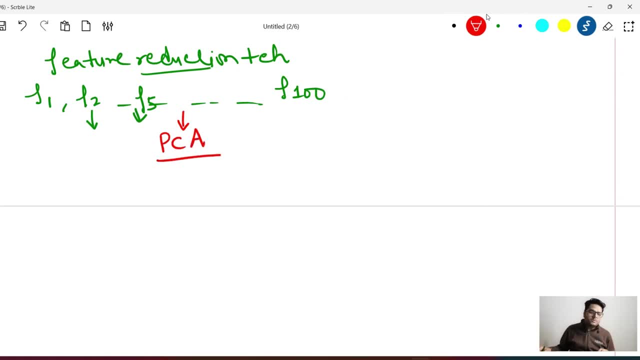 standing for principal component analysis. so what PCA does, if you take your data and if you apply a principal component analysis on your data, all these features right, what PCA will give you is: PCA will give you principal components. we will understand in detail what is principal components for now. I am telling you for these hundred 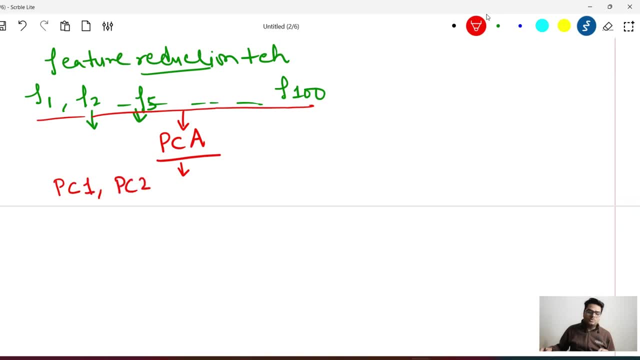 features. PCA will give you 100 principal components. ok. one more interview question, guys: how many principal components for hundred features? ok, 100 principal components by default. out of these hundred principal components, what PCA tells you is: you no need to consider all these hundred principal components for your model training. rather, you can consider top. 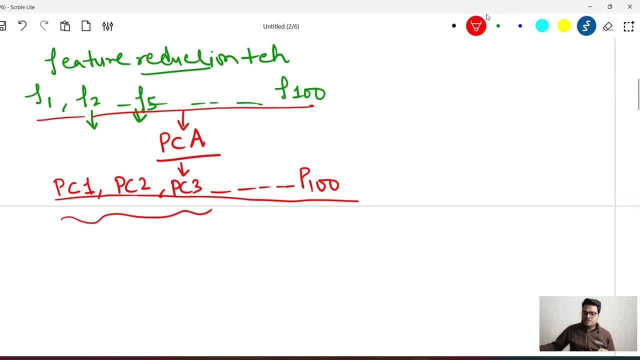 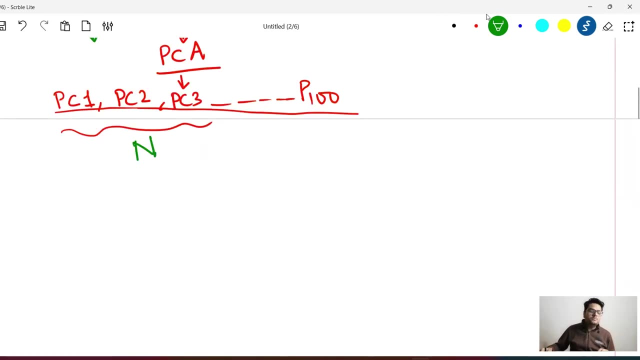 let's say n features, Top n features. features on the basis of what I will select. top end features on the basis of how much of my data variance is explained by these features. So how it works generally is your PC1 will explain most percentage of your variable in. 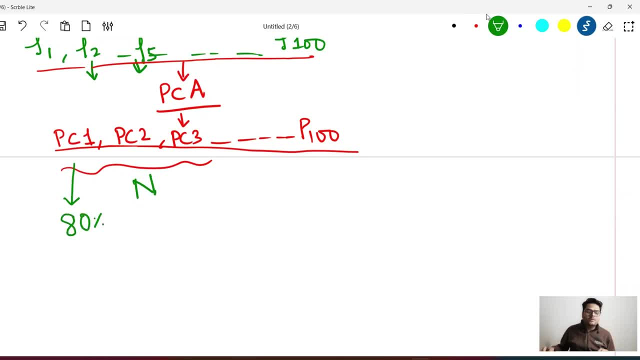 your data. So 80% of your data will be explained by PC1. Another, let's say 15%, will be explained by PC2.. Another 3% will be explained by PC3. And whatever is left will be explained by another principal components. 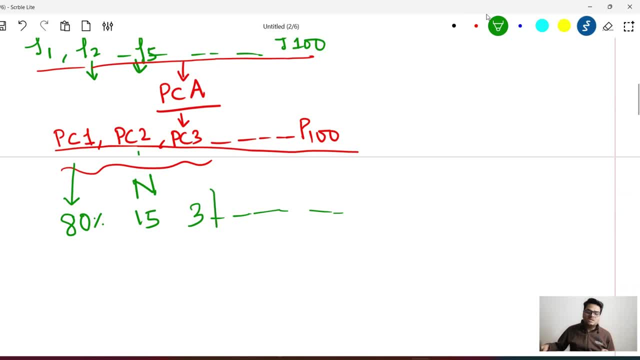 So you no need to take you know anything after PC3 in this case, because if you see 95 plus 93, right, 98% of your data variance is explained by first three components only. So from 100 features you have come down to three principal components and you are losing. 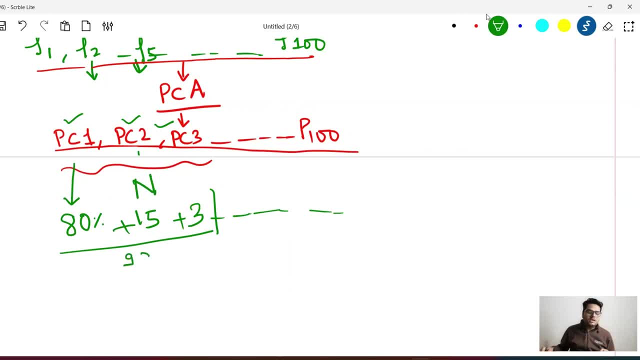 just 2% of information of your data, because 98% is being explained Now. it's not very simple, guys, reducing your hundred features to three features. It is complex mathematics behind it, and hence I have broken it into multiple pieces. We will go one by one. 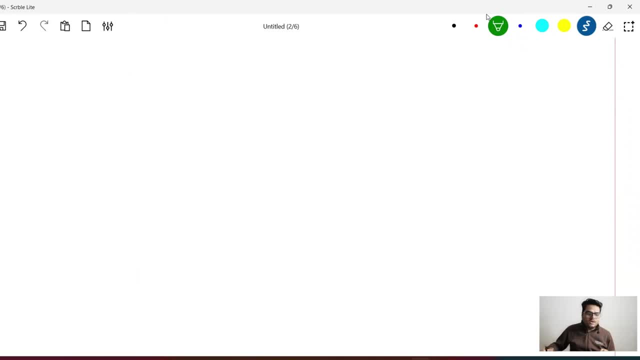 So first of all, guys, few basic, fundamental things we will discuss. I hope you know what is the difference between a scalar quantity and a vector quantity. If not, let me give you a small examples. Anything where you see only magnitude, it is a scalar quantity. and anything where you see 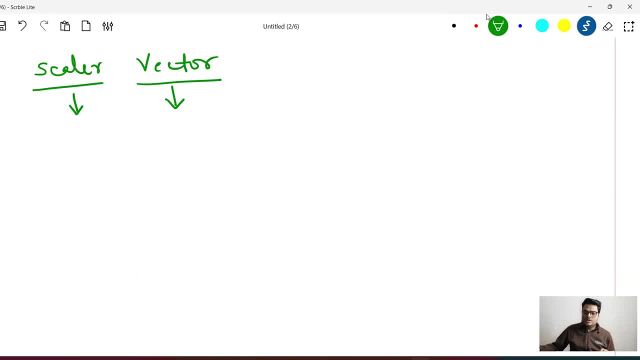 magnitude and direction, both. it is a vector quantity. For example, if I tell you what is my weight, okay, weight does not have a direction, just a magnitude. So it is a scalar quantity and vector quantity example. let me give you, like this: Suppose: there is a aeroplane flying, okay, and this is your x axis and this is your y axis. 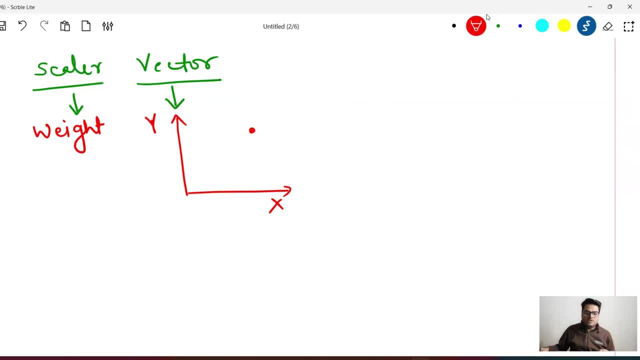 now somebody asks you what is the position of the aircraft. let's say this is three units on x axis and four units on y axis. Somebody asks you what is the position of the aircraft? you can say something like three, four. okay, this is the magnitude, but in which direction this magnitude is there? 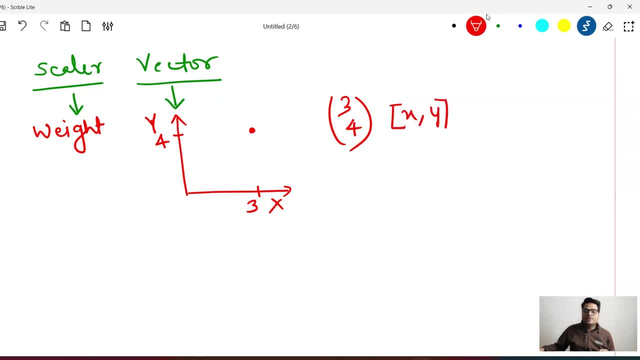 So direction? you will say like this: x, y. so in x, y direction the respective magnitudes are 3 and 4.. So what we are discussing here? we are discussing here a magnitude and a direction. So this is a vector quantity simple. let's move on to next mathematical concept known. 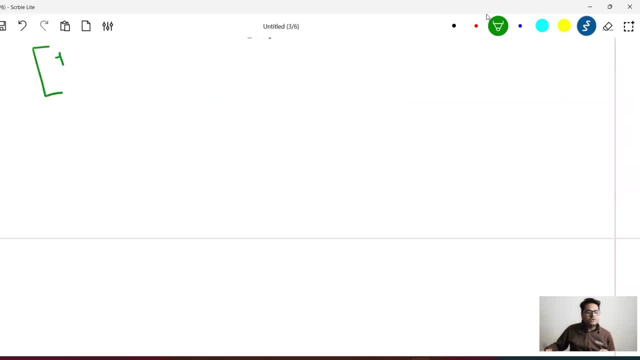 as matrix. So in mathematics, guys, if you write few numbers like this, right, this is a matrix. you know this already. okay, and what is the matrix transpose, guys, if I apply a transpose on this matrix, then this will be like: rows will convert into columns, columns will convert into rows. 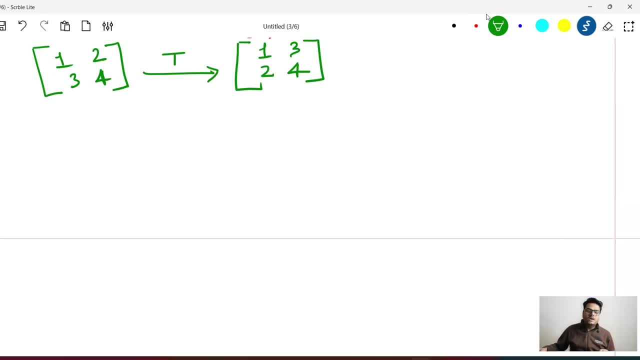 This becomes your matrix transpose. okay, I am sure you know matrix multiplication, just, but just little. you know detail. I will do a simple matrix multiplication. If I have to multiply this matrix A with the below matrix B, right, how the multiplication will happen is it will go like this: you have to go in first matrix, row wise second matrix. 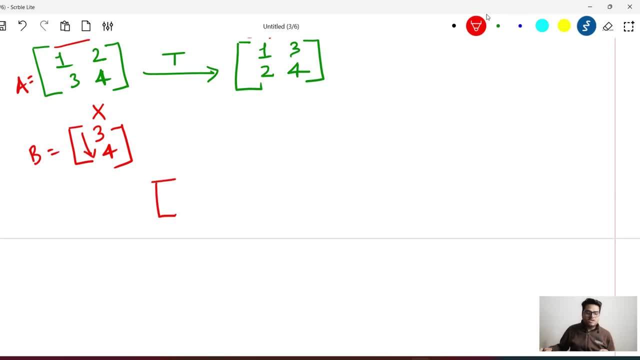 column wise, okay. so the result of this matrix multiplication will be: one gets multiplied with three And two gets multiplied with four. this becomes one element of your multiplication matrix. again, three gets multiplied by three and your four gets multiplied by four. that is your another element in the matrix for matrix multiplication. remember, guys, the dimensions would match. so 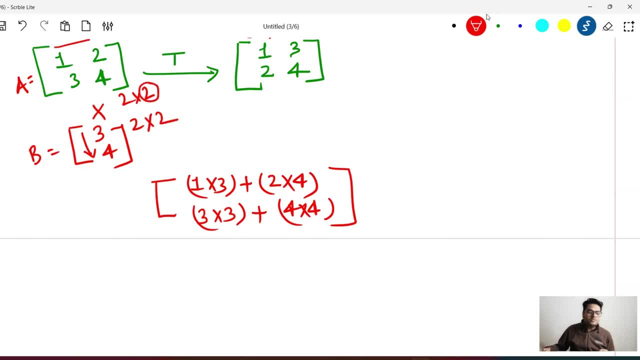 if I am considering row wise here, then row is two. this should match number of columns here. am I saying other way around? number of columns here should match number of rows here. Yeah, so number of columns here two and number of rows here too. So both these things would match. you already know this. just a refresher, okay. 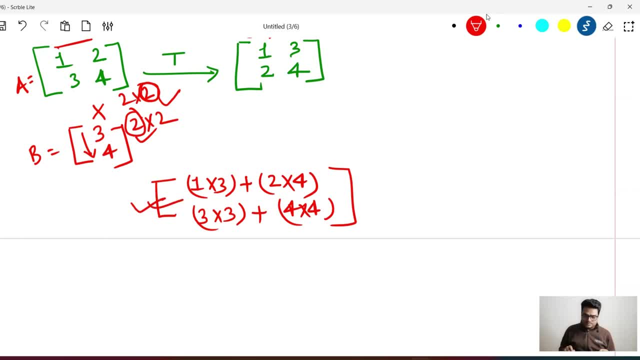 So this is your multiplication product. Now, what I am going to do is I am going to tell you the concept of something known as eigenvalues and eigenvectors. okay, So you saw one matrix. guys, let us call that matrix as matrix A, for any matrix A. okay, understand. 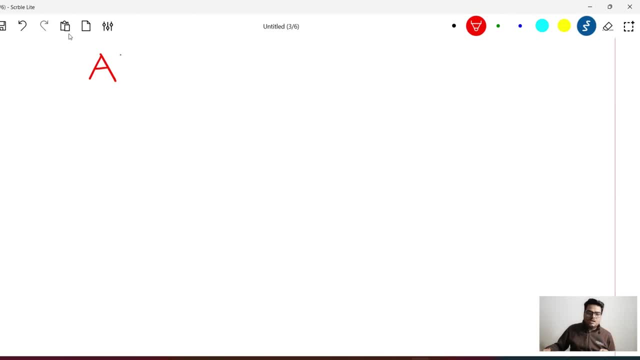 this carefully, guys: for any matrix A, if there is a vector V, such that if I multiply that vector with a scalar quantity then this equation becomes true, then this lambda is called eigenvalue- okay, for that matrix A. and this V is called eigenvector for this matrix A. one more time: 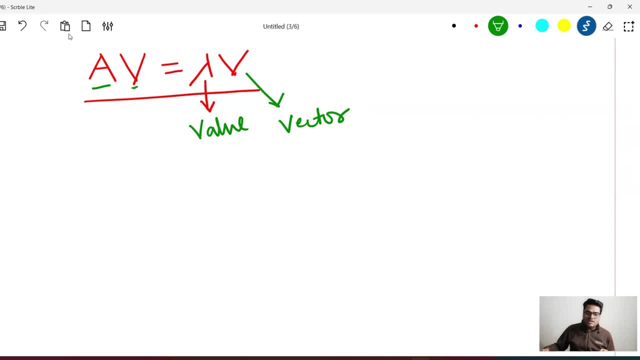 guys. So if I multiply this matrix A with this vector V, then the results are the same. then this lambda is called eigenvalue and this vector is called eigenvector for this matrix. One example, it will be absolutely clear: Suppose there is a matrix, simple matrix. guys, I will write here: three, six, five, four, okay. 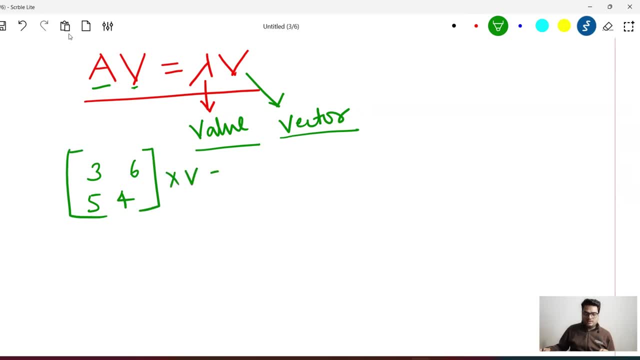 and if this gets multiplied with a vector? Okay, And if lambda gets multiplied with a vector? Now suppose I want to find out what are the eigenvalues and eigenvectors for this matrix. okay, So what I have to do is I have to solve a quadratic equation, basically. 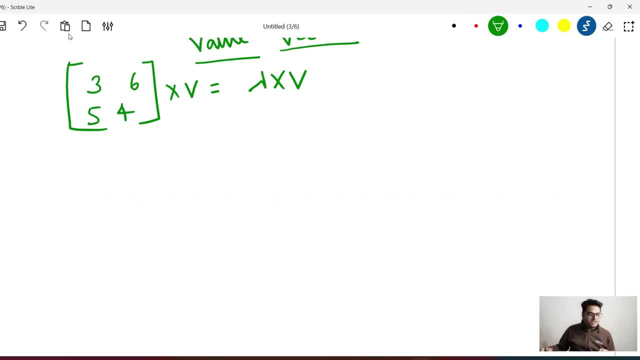 So how it will be solved is: you can just bring this- you know this right hand side term here- and equate it to zero, and if you take the V out, then you will see that inside we have our matrix okay, and then we have our minus lambda. I. 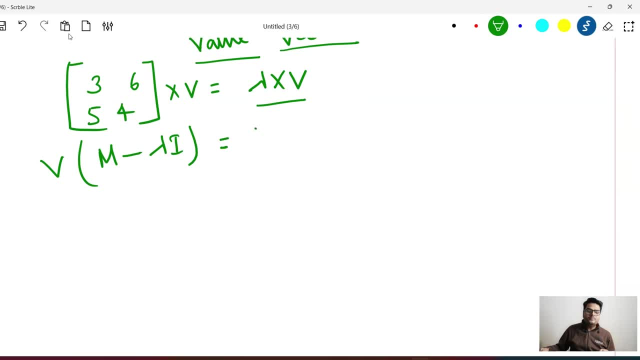 Okay, I is nothing. but your identity matrix, okay, is equal to zero, assuming V is a nonzero quantity. if you solve this equation right, you get the value of lambda first. So your matrix is what? three, six, five, four, right? and you are multiplying with lambda identity. 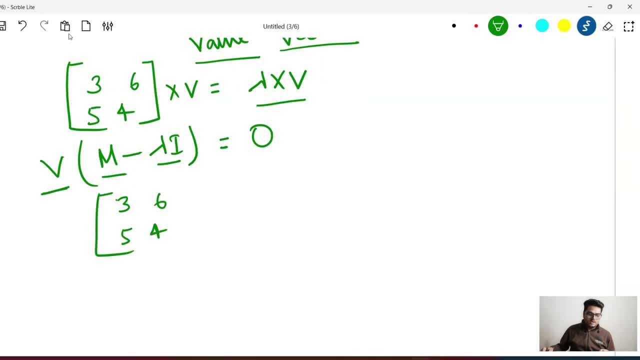 So let me write it here. maybe some people might not be able to get if I tell like this lambda into identity means your identity matrix is nothing but a matrix of one, zero, zero, one. okay, So the main diagonals will be one, other will be zero. 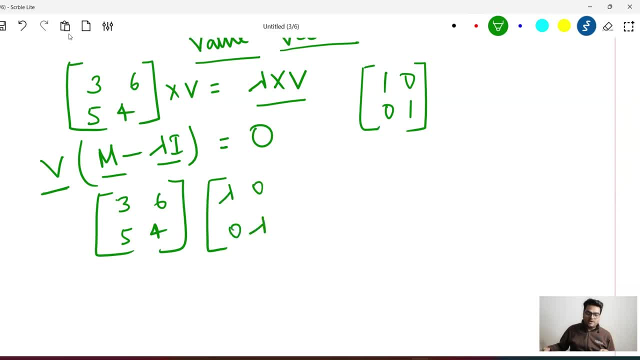 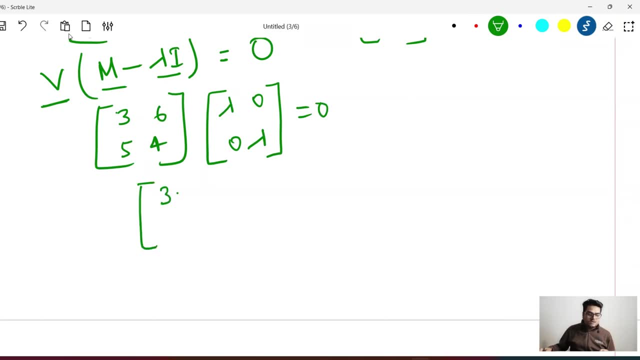 So if I multiply lambda with that, then what happens? lambda zero, zero lambda, This is equal to zero. Now what is this? if you subtract two matrices, three minus lambda six, five minus zero, four minus lambda zero. Now if you want to solve this: three minus lambda multiplied by four minus lambda minus. 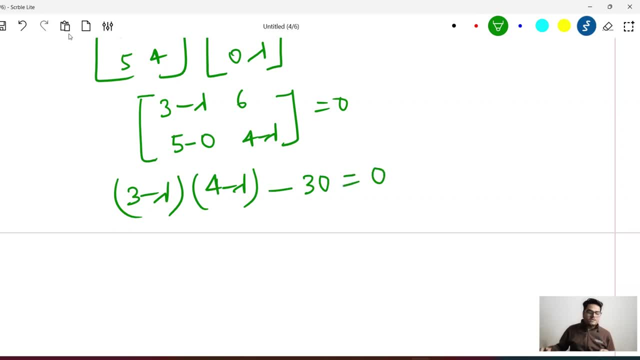 30 is equal to zero. okay, and this is nothing but a quadratic equation, guys. and if I solve this quadratic equation, I'm seeing in my notes, you get two values of lambda: one is nine and other is minus two. Now, important thing to understand here, guys: I told you the definition of eigenvalue and 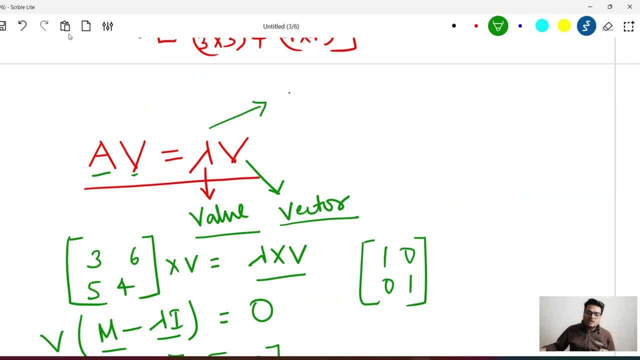 eigenvector. So how many lambda values? I'm talking here? nine and minus two. Two different lambda values means two different eigenvalues. So how many vectors will be here? One vector will be associated with this. one vector will be associated with this, okay. 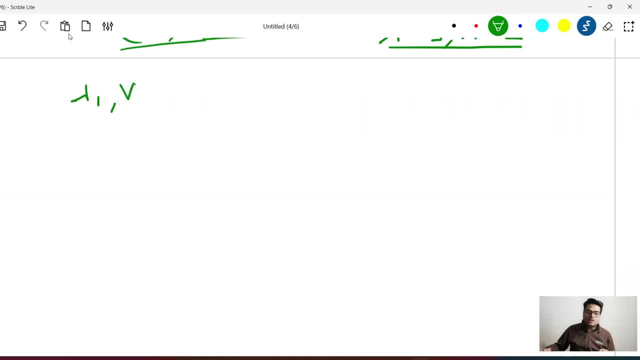 So in the end you will have lambda one v one, one combination. lambda two v two- other combination. Now why we are doing all this calculation and why it is extremely, extremely important concept in mathematics. If you see here carefully, guys, Let's see, Let's see. 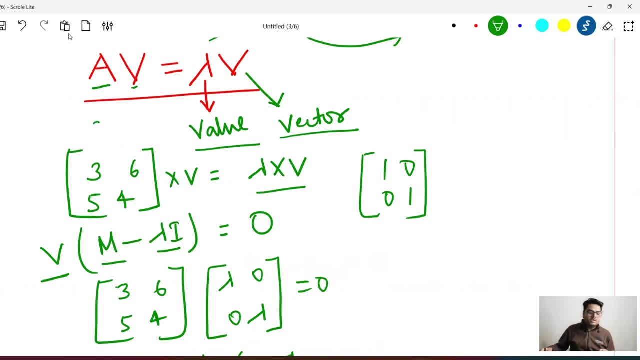 Our, our matrix right, which is a two cross, two matrix. we are able to represent this matrix by a vector, which means we are bringing it to a lower dimension. okay, and lower dimensions mean nothing but dimensionality reduction. So what we are doing here is we are trying to see in which direction maximum variance. 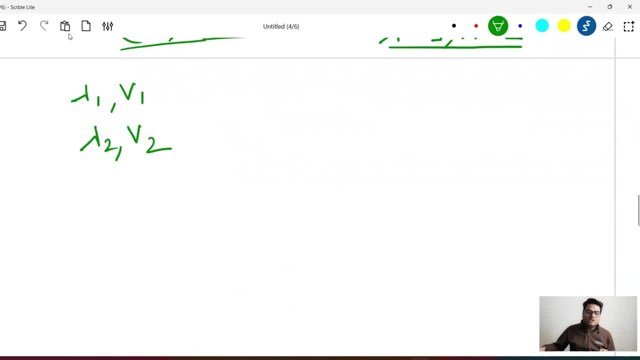 is there in the data. data means matrix in this case. So, for example, If this is your vector, one, okay. So vector is what? your direction? Remember this, guys understand this. your your vector, else the direction: okay. and your lambda value, which is your eigenvalue, tells you what is the magnitude in that direction. 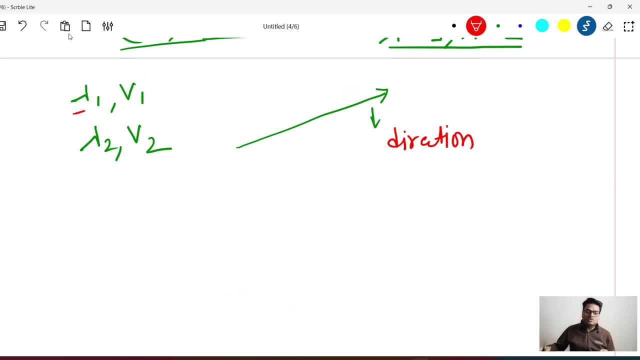 So I understood the direction. but what is the magnitude? So your lambda value is one value is nine and one value is minus two, right, So this is your magnitude in this direction. Okay, This is the mathematical intuition behind something known as even value and even vector. 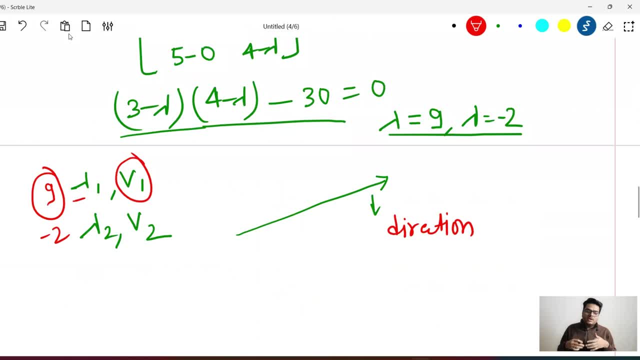 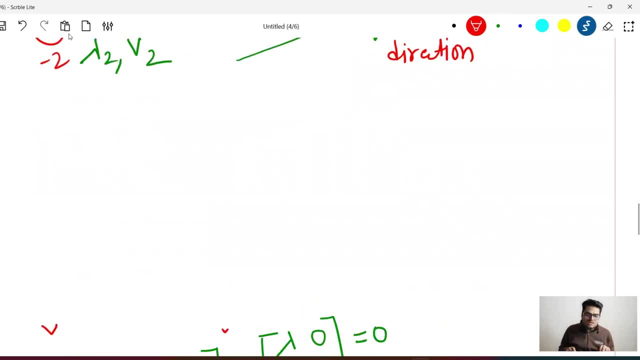 We are decomposing this matrix in a lower dimensional space and we are knowing in which direction, how much is the magnitude. fine, after this, what we will understand is how to compute. we have done all the raw work. now how to compute PCA step by step. okay. 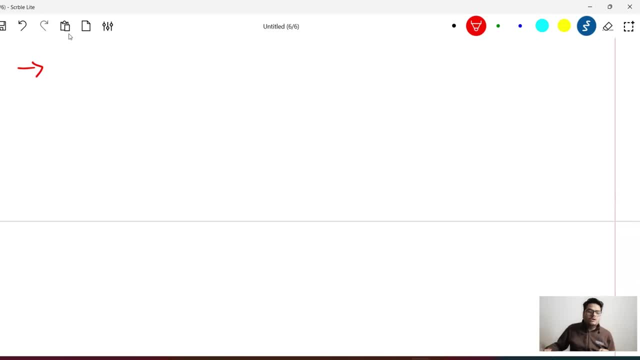 So suppose, guys, I take a very simple data here. okay, I take marks of two students. okay, physics, I will write here physics and I will write here maths. okay, this is my student one, this is my student two. so student one scores some a marks. student one scores in maths b marks, c marks and d marks. right, I will take this. 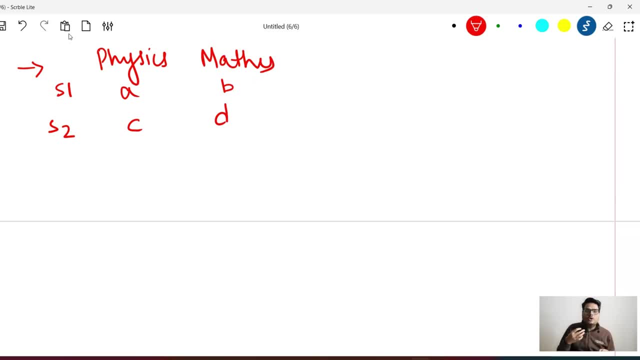 simple data and I will tell you, step by step, how PCA is calculated when you call sklearn PCA First of all. So let me show you what happen is. this is step one. let me take a different color. this is your step one. what you have to do is: first thing you have to do is you have to define. 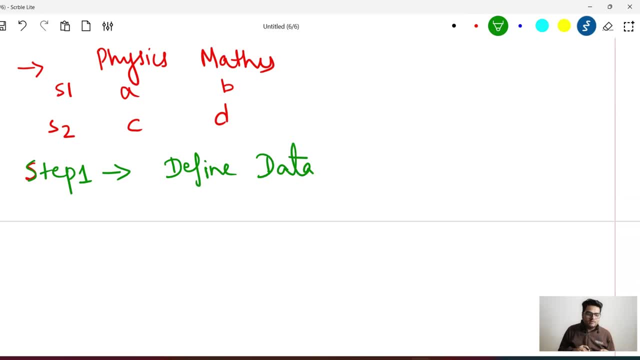 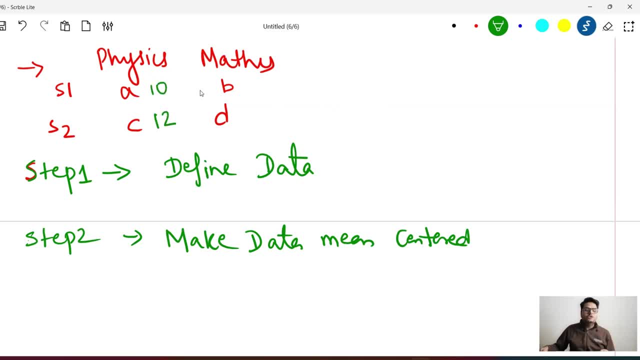 guy scores 10 marks, this guy scores 12 marks. okay, so, feature by feature. this is your one feature, right? this is your other feature, right? feature by feature, we want to kind of scale the data. in this case we are doing the mean centering based scaling. okay, that is the step two. and now? 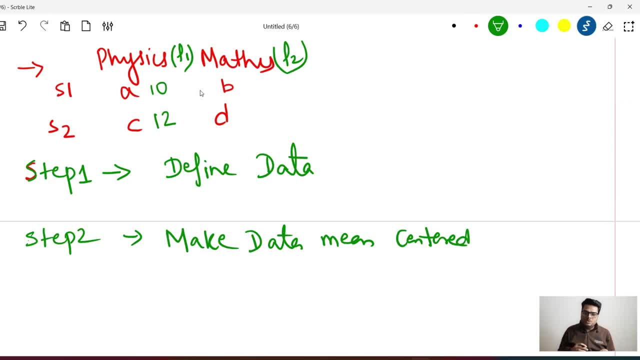 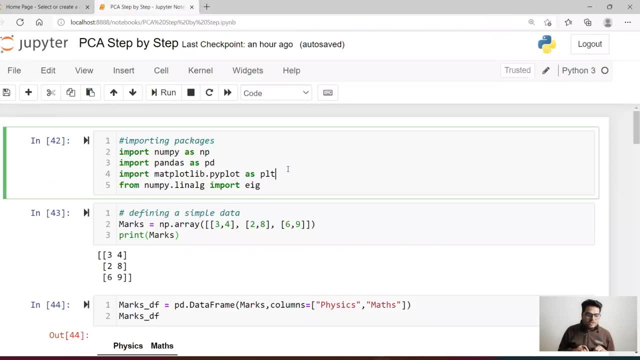 i will take you, i will tell you one step and take you to the python notebook also. so, guys, if you can see here, let me go to my jupyter notebook. okay, as you can see here, import numpy pandas, matplotlib and from numpy dot linear algebra. i am importing egan, so i will tell. 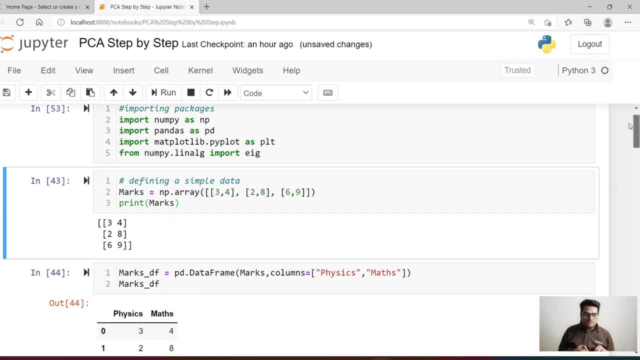 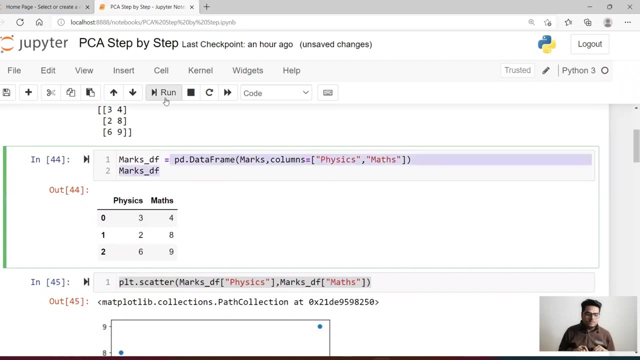 you what it does, like the way i was saying. you i have, i have defined a marks data here and these are the marks of the students. okay, in three different students in two different subjects. you can say okay, and i am kind of creating a period or data frame, i am giving the column names. 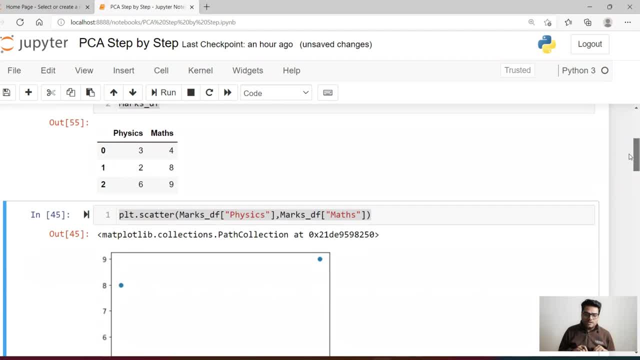 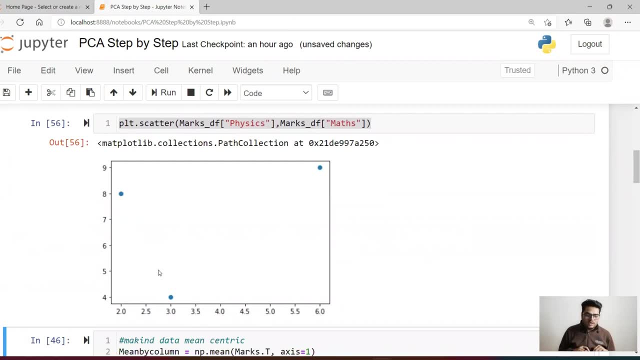 all those things you know already and if i am plotting this, then it will look like this in the beginning. now see these guys in the beginning. this is the how data is scattered okay, and what we are trying to do. we are trying to capture the, the direction in which maximum variance of the 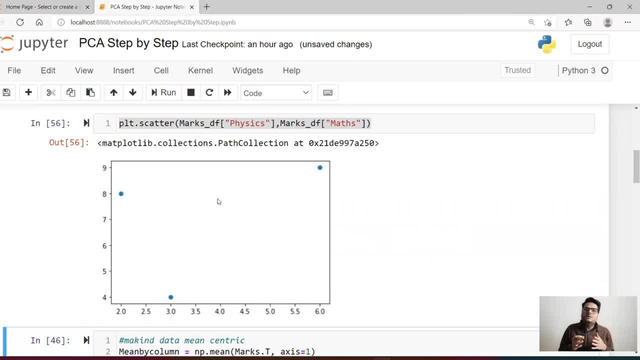 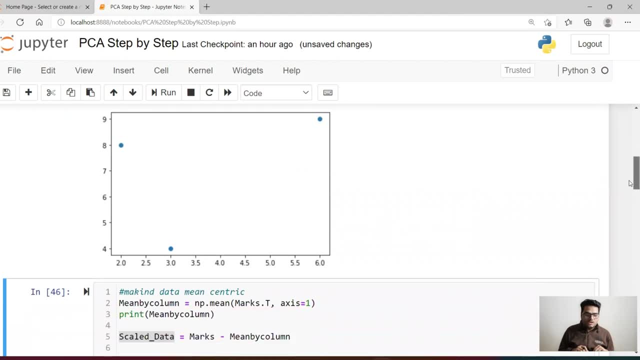 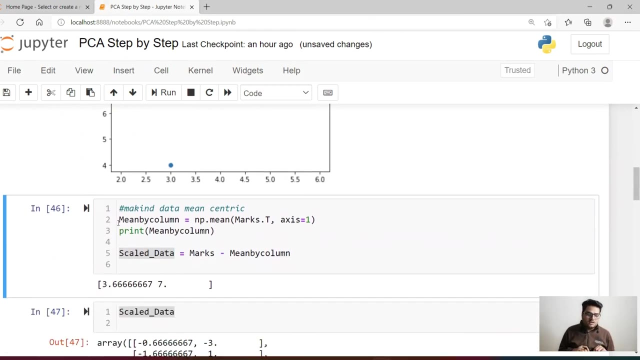 data is there. so, by looking at this, in which direction you think the maximum variance is there? guys, obviously not in original x, y direction. maximum variance is there. okay, so we will see how to do. do that right one by one. so i was talking about making data mean centric, so what? 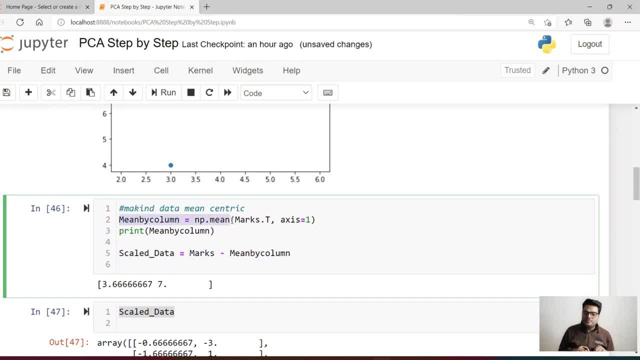 what i'm doing here, mean by column, is equal to numpy dot mean marks dot. transpose now why we are transposing. every time i say dot, t means i'm transposing. so if you want to see what is in marks, transpose guys. uh, it is nothing but your transposed data, okay. 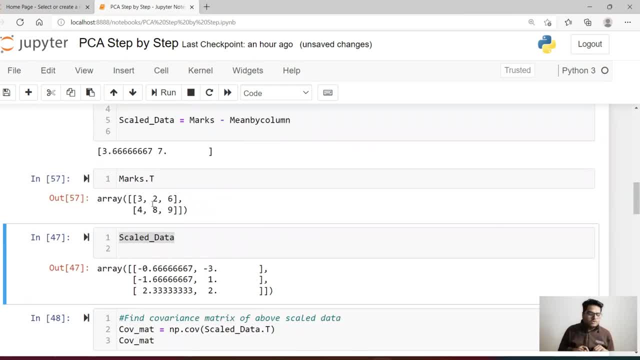 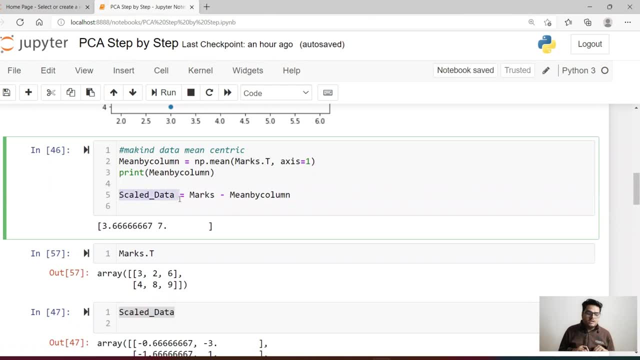 because i want to take the mean column. wise, right. so three, two, six comes here and four, eight, nine comes here and i want to take the mean and then i'm i'm scaling the data by subtracting mean by column. okay, so if you see, here i'm printing mean of each column and my scale data will look little. 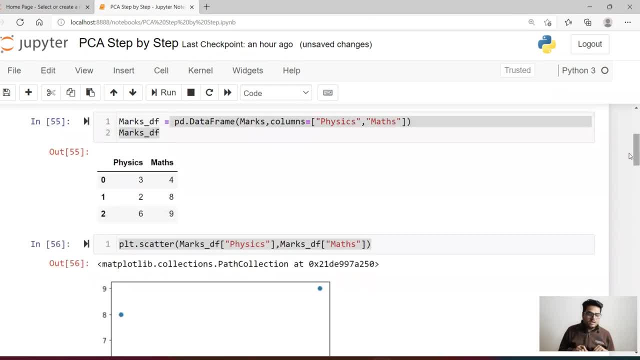 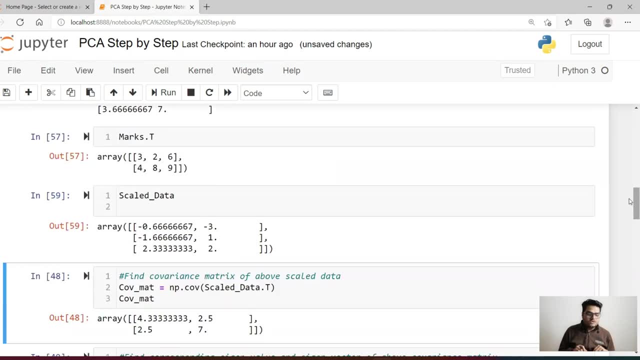 different than the original data. for example, the original data is like three, two, six, four, eight, nine- i take the mean subtract from all- and if you see here, the numbers of data will be changed. okay, this is scaling. why scaling is needed? because we will be doing everything on the axis and rotation will happen. so imagine if one of your data is on bigger. 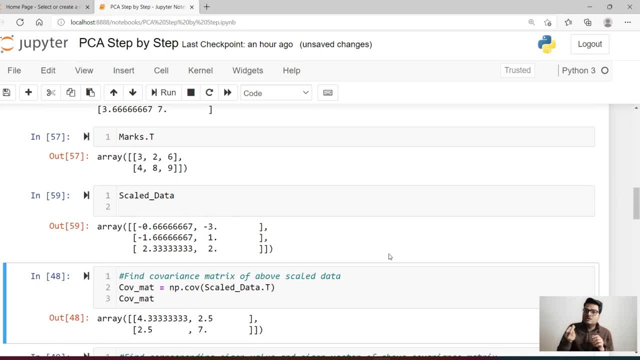 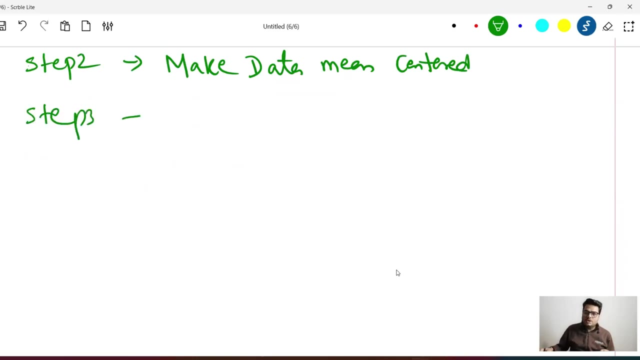 dimension or axis, not dimension. bigger i mean to say magnitude other is on a smaller, it will be a problem. so we are doing this. next thing. what we have to do is we have done the data. mean centric, okay, in step three. mean centric purpose. you would have understood, i'm sure. um, in step three. what we have to do is we started with. 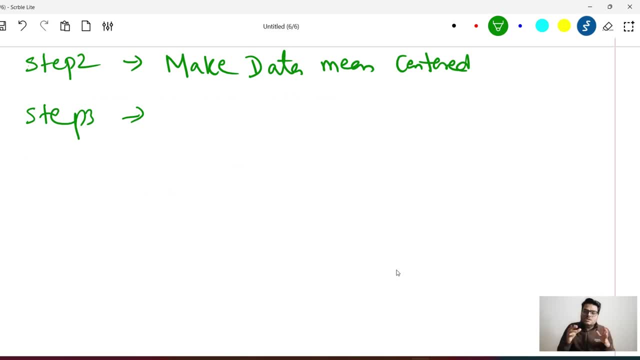 many features in the data right, and now we want to understand which features are related to each other more and which features are related to each other less. that is the whole purpose of dimension reduction, right. we want to understand that. so in step three, we are going to create something known. 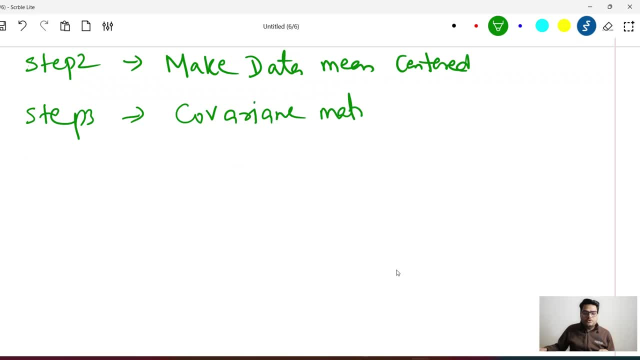 as covariance matrix. if you forgot this concept or if you want to revise this concept, i'm giving a link here, guys, for one video. you must watch that video. covariance is nothing but another, uh measure to see how two variables are varying together. okay, so in covariance matrix. 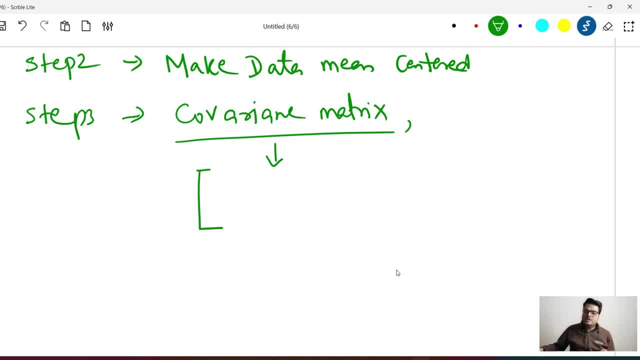 what you will see is if i have to compute covariant matrix between two features, a and b, right, so it will be covariance between a and a, covariance between a and b, covariance between uh, b and a, again between b and b, something like this. so it will give you covariance numbers in different dimensions. 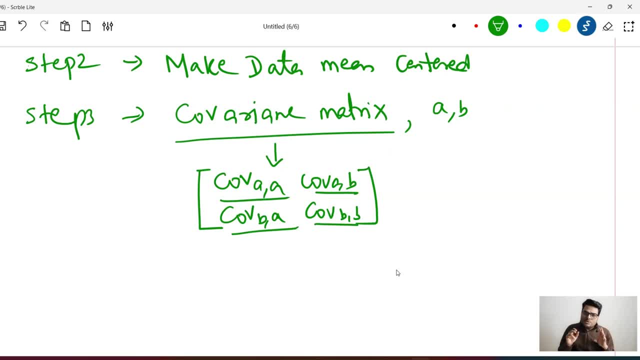 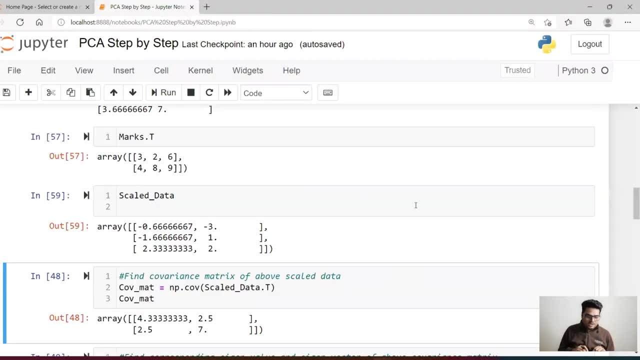 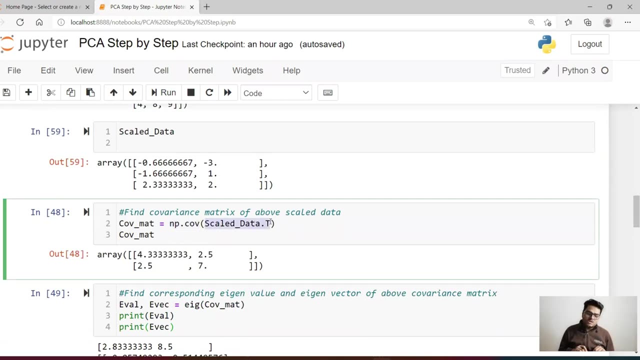 in a matrix format. why it is needed. we want to understand relation between different variables. okay, how to do that in python? let's come here again. and covariance is nothing. but you just go to numpy and say np, dot, cove scale, data, dot, transpose. again, because we want to do it feature. 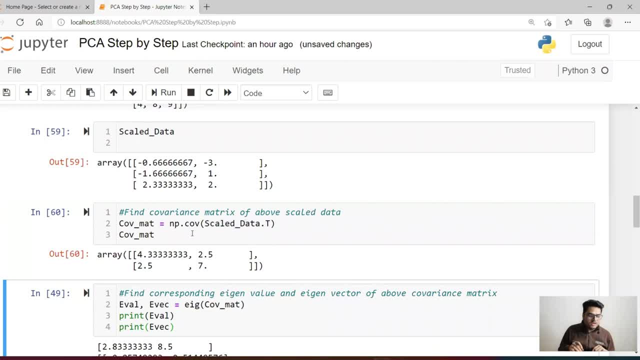 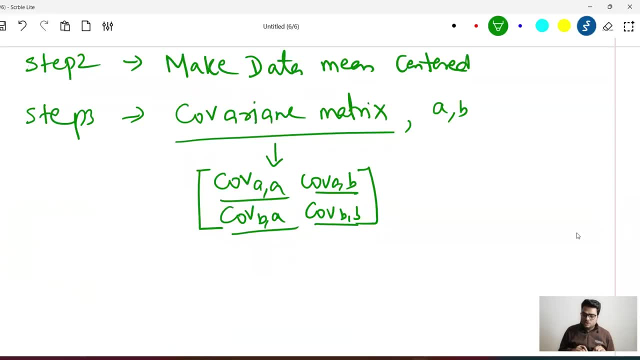 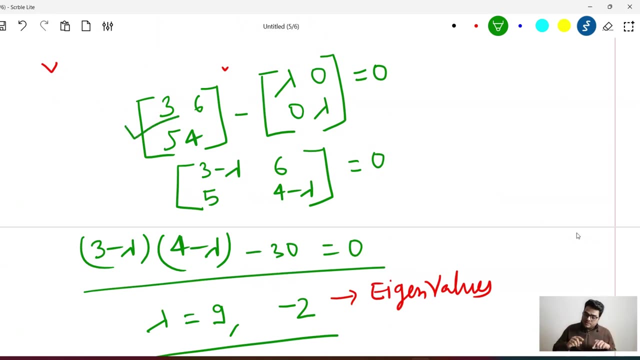 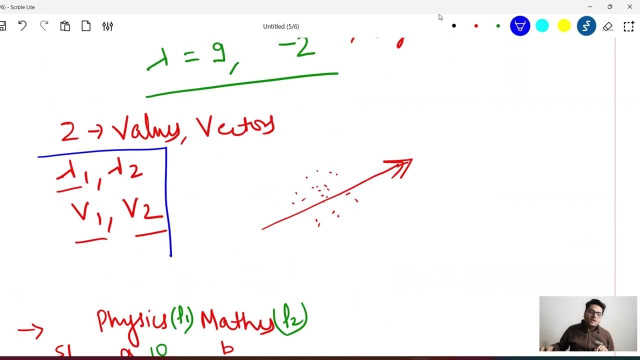 by feature. okay, so this is your covariance matrix. once you have the covariance matrix matrix, the next step is nothing but what i explained you, using even value and eigenvectors. now your covariance matrix become this matrix and what you have to find out is corresponding lambda values and v values. what we want to capture, guys, for that covariance matrix, what is the direction? 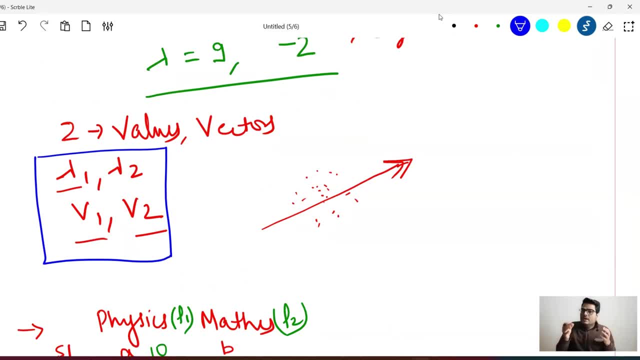 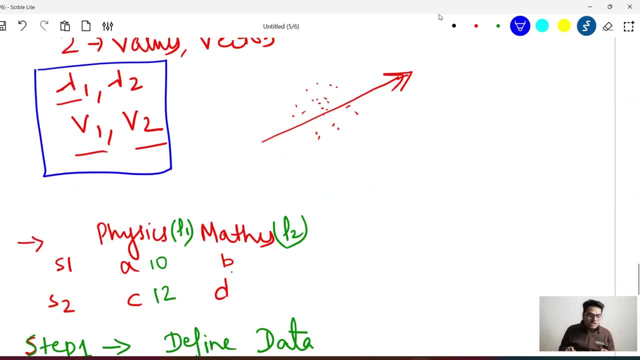 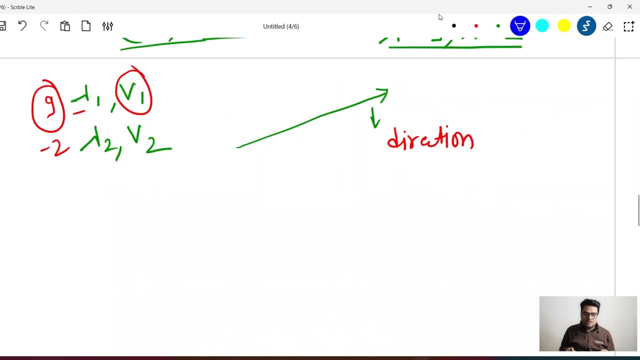 in which my maximum variance is there, and also what is the magnitude in that direction in which my maximum variance is there, and also what is the magnitude in that direction where the variance is or how the variance is. so, uh, we did all these calculations manually here, just to show you. i showed you right. matrix, subtraction, finding of lambda, all these things. 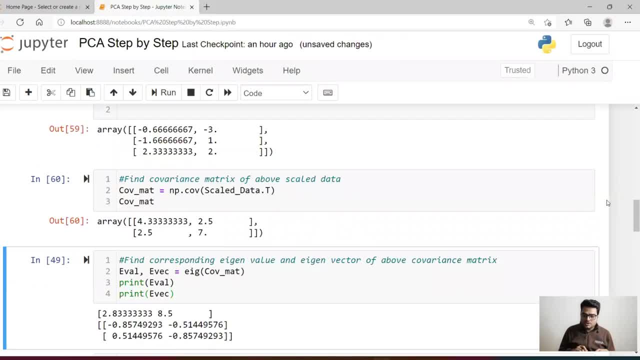 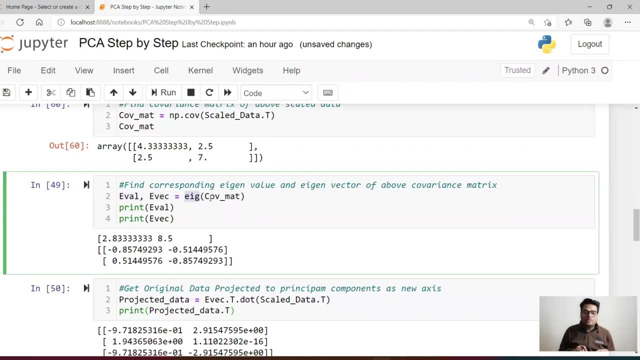 in python, all these things will happen in one shot. you come here and you say: eval means eigenvalues, evac means eigenvectors. you just say ig of covariance matrix. so the first thing that you can see here is your eigenvalue, second thing that you can. so this is your lambda. 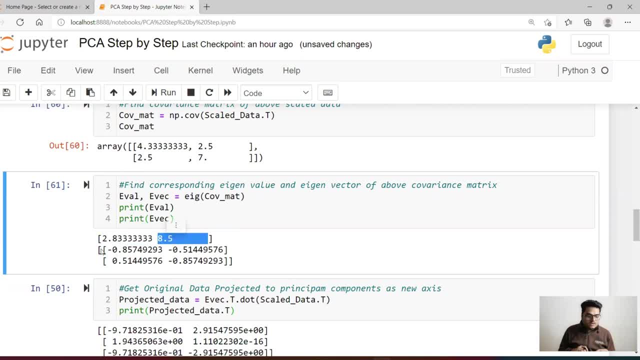 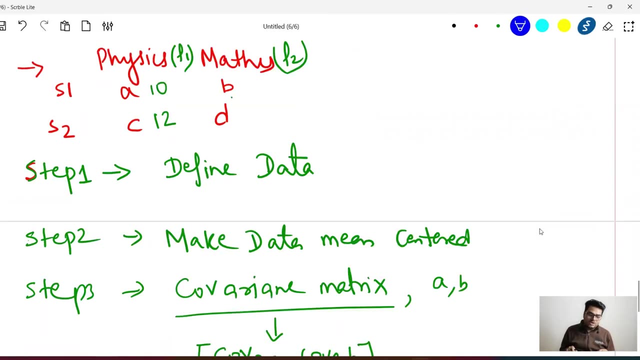 one, eight. point five is your lambda two, the, the second thing which you can see here. this is your eigenvalue, i'm sorry. eigenvectors first, eigenvector second. so lambda one, lambda two, v one, b two you are having here. okay, so once you have the lambda one, lambda two and v one and v two. 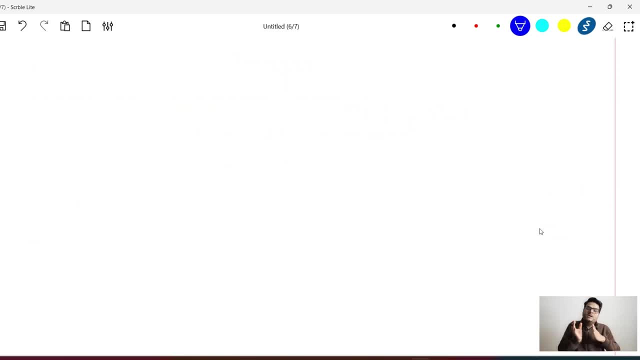 then what you know is where your covariance matrix direction is and what is the amount of magnitude. but you do not want to work on the um. you know lambda one, lambda two and v one and v two and V's. only You want to project your original data to that axis. For example, let's say there: 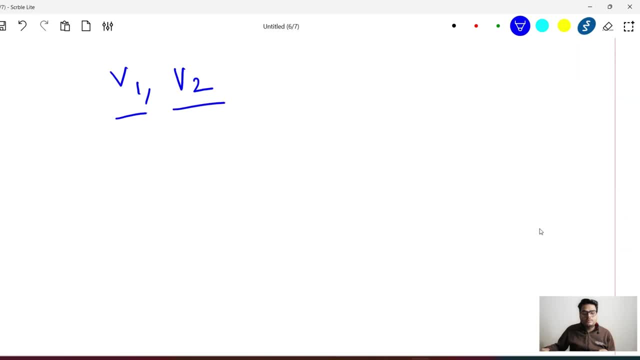 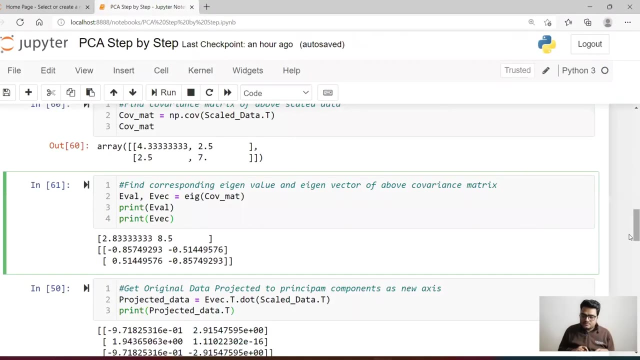 are two vectors. in these two directions, your spread of data, or variance, is maximum. What you want to do is you want to move your original data to that scale. Okay, So your original data here in this case is this right: 3,, 2,, 6, or 4,, 8,, 9,, or even if you take your scale data right. 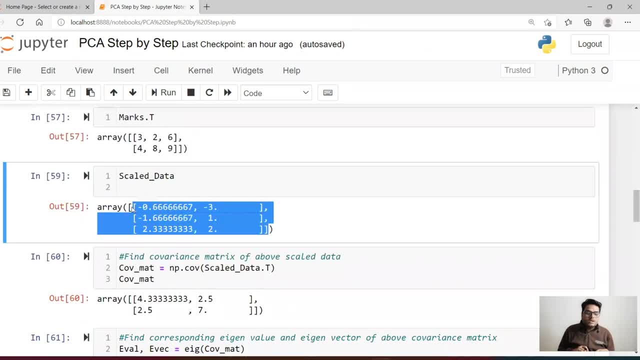 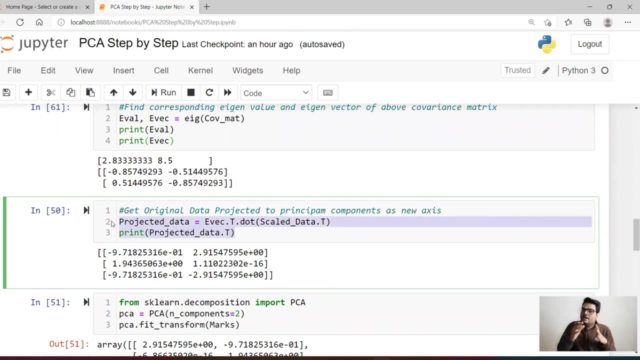 that is your scale data which I showed you here. Okay, This needs to move to the new axis. New axis means new vectors. New vectors means I will come here and tell, hey, can you project my data to the new, new axis? So how I do that? I just go and say again: vector transpose. 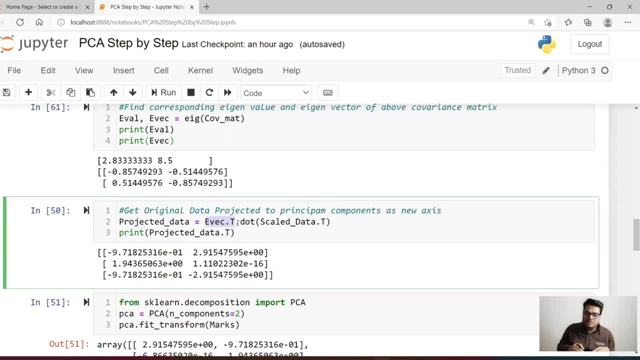 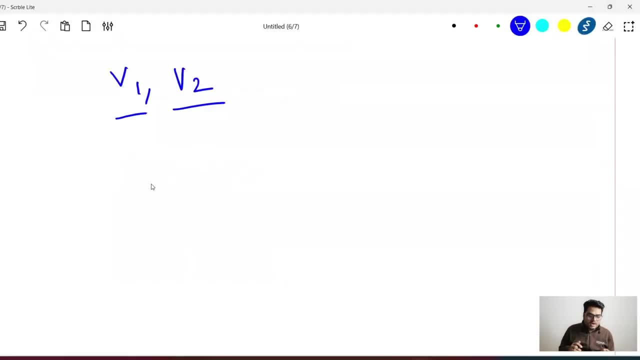 because that that vector is there right- V1, V2 I'm talking about- and take the dot product with scaled data, transpose, Okay. So what I'm doing here, guys, I'm kind of projecting original data. project. original data to new axis, project. original data to new axis- Okay. And after 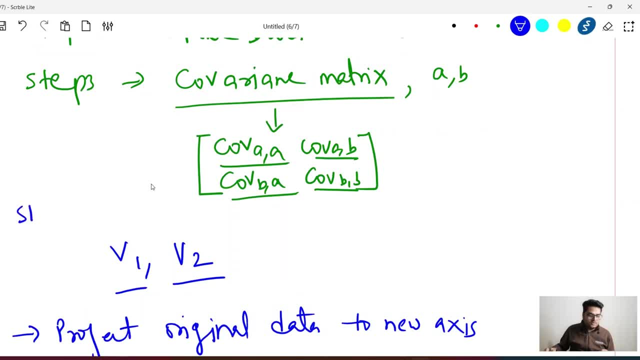 after you create this, then you'll find in step four, then you'll find lambda one, lambda two. Okay, Find even values and even vectors. that is lambda one, lambda two, V1,, V2.. And this is your step five, Once you find your. 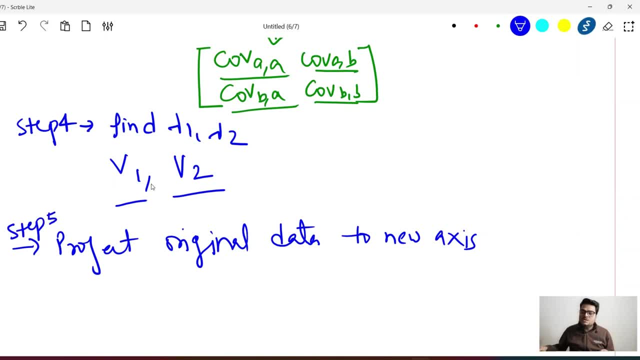 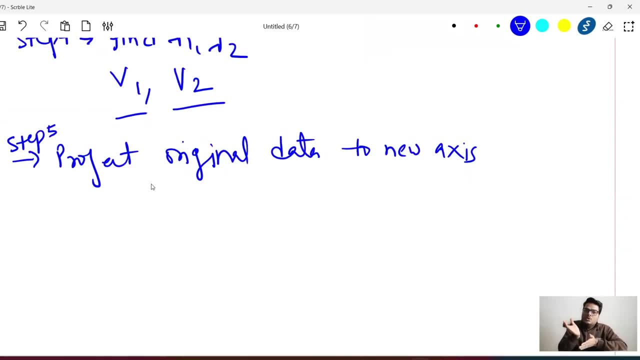 lambda one, lambda two, V1, V2,. then you project your original data to the new axis because you you have found the direction of the maximum variance. Now you do not want to use the old axis because you want to use the new axis where you want to project. 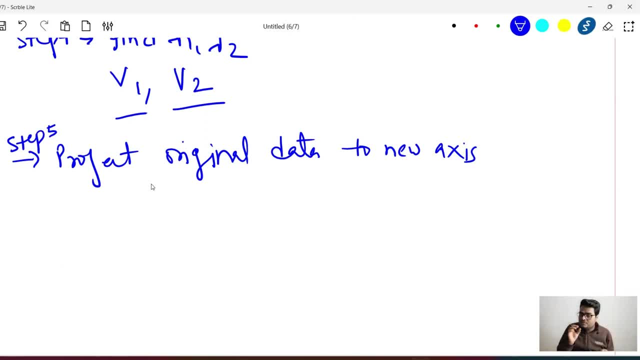 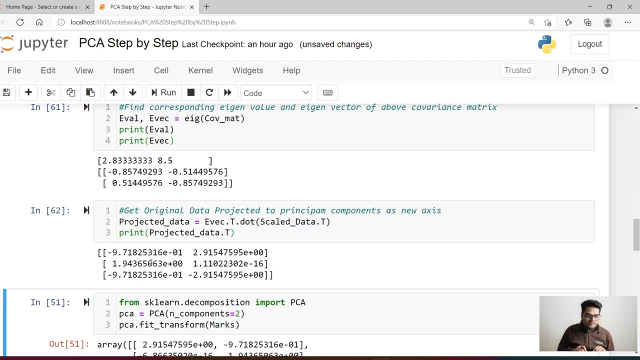 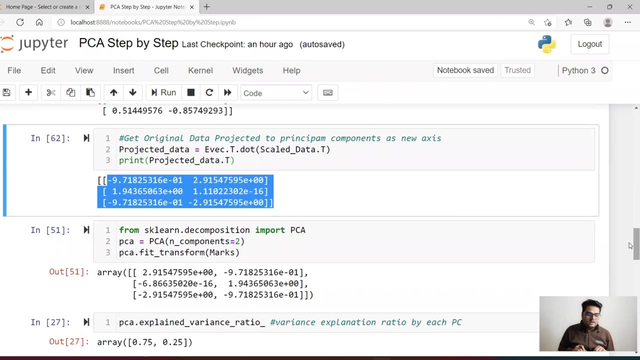 your new data and use that because you want to use limited number of vectors or principal components, right, So it will give you. once I run this, it gives you these values And what I'm highlighting here is nothing but your principal components. Okay, And in this line, 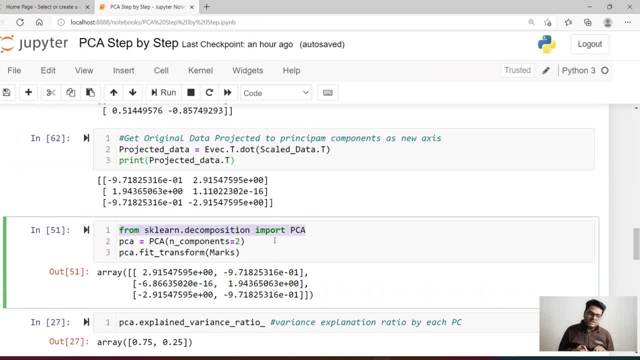 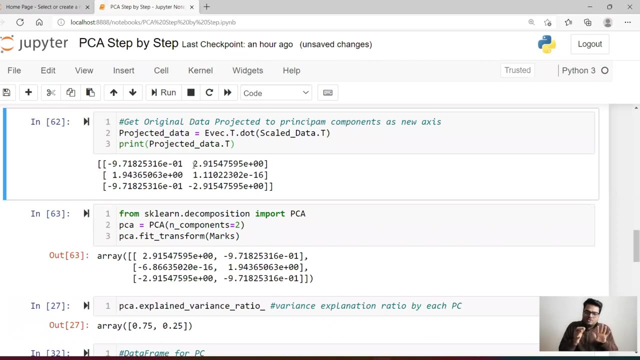 what I'm doing here. I'm importing from a scale and decomposition import PCA. I'm running the same thing on marks- original marks, not scaled or anything. Okay, And if you compare the results, guys, you see that the numbers look absolutely same. For example, the vectors are swept, So don't. 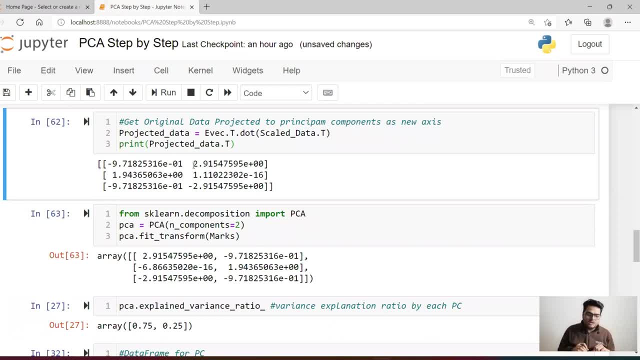 bother about that, Don't bother about the signs. also, just see the magnitude. Okay, 2.9154.. This is the main one here. This is the main one. Okay, And here another vector. Let me run this again. Let me run this again. Did I miss any step in between? Okay, Yeah, This is your 16 zeros, So. 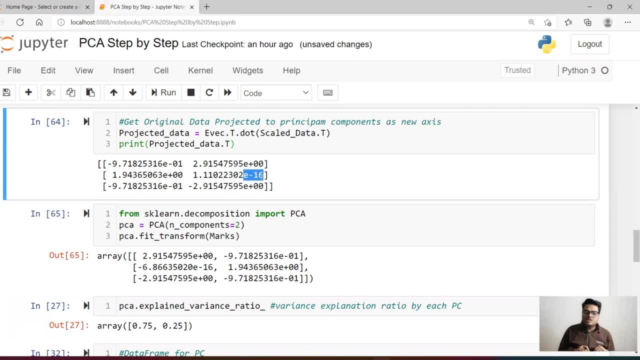 this does not matter, Guys. e minus 16 means 16 zeros. This is a very, very, very small number And we don't bother about this. This is 1.11.. And this is 6.86.. Very, very small 16 zeros. Okay, Main ones are 2.91, because 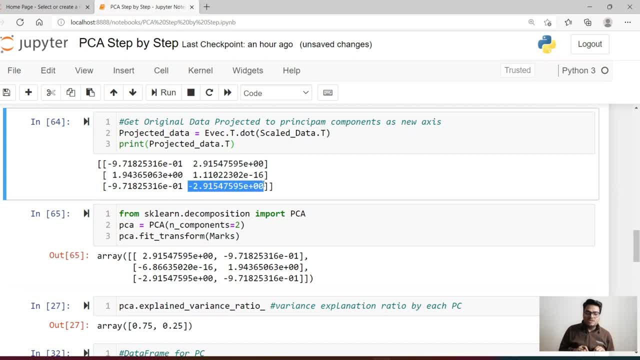 there are. there are no much zeros and minus 2.91.. No much zeros. Okay, Let us compare the second principal component, Second principal component: minus 9.71 e minus one. minus zero one: 1.94, 1.94, 9.71, 9.71.. 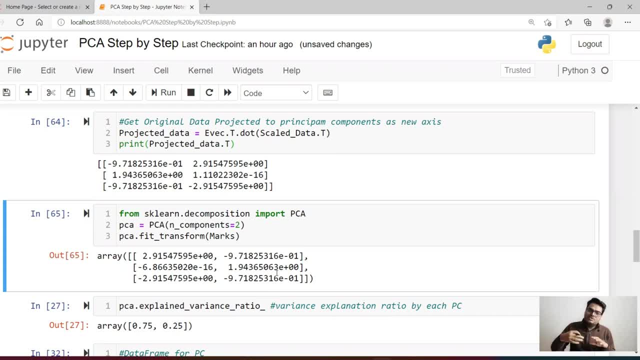 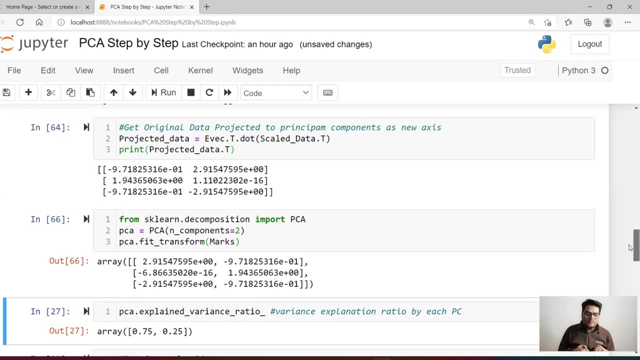 If you leave some decimal margins, which is after so many decimals, right. Exactly same results, guys. just the lambdas are swept. which means it is considering this vector as the first vector. manual calculation considering other vector as the first vector. So this is how you compute PCA by: 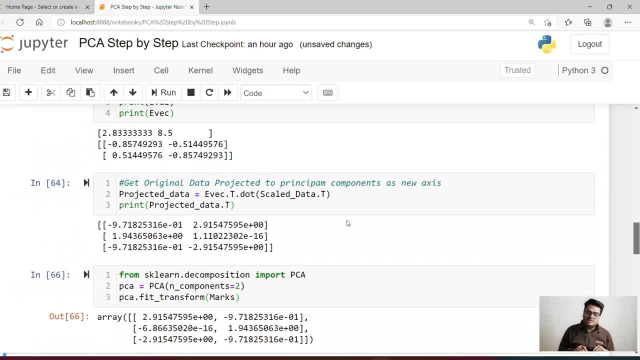 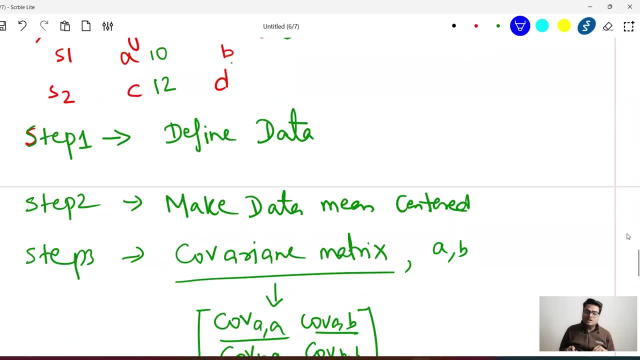 manual process And the result is same as your SQL and PCA. Okay, one more time. what are the steps? First of all, you have to compute the. we have to define data, make it simple, and then you have to compute it. And then you have to compute it, And then you have. 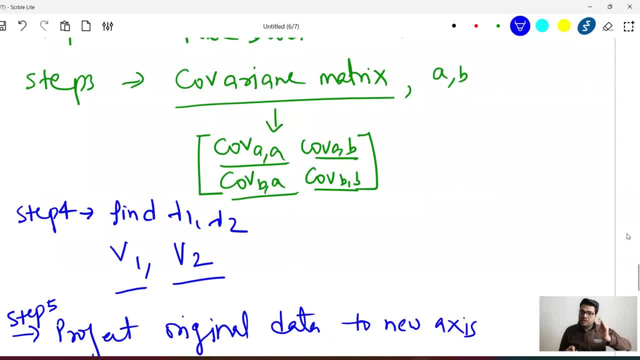 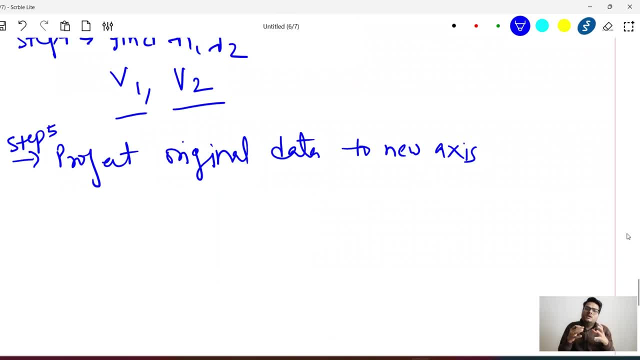 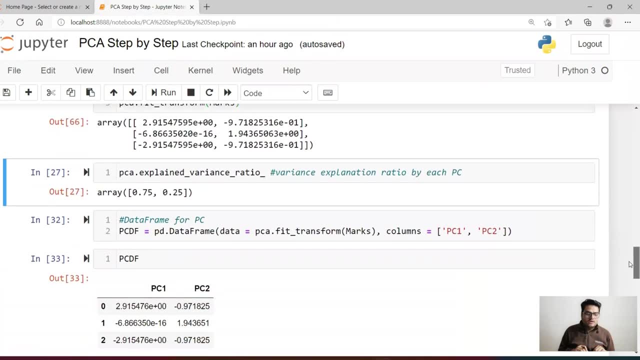 dimension and direction. Okay, how you do that. you multiply with the scale data with these vectors. Okay now few important things here, guys. So explained, variance tells you how much is the data in your data. how much, why, do you think? explained by a first principal component. 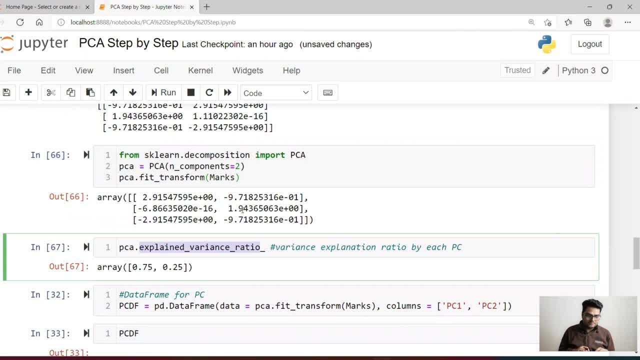 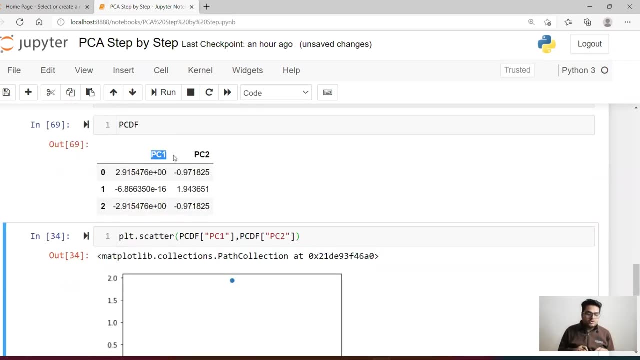 and how much variance is explained by second principal component. In this case, 75% variance is explained by first principal component, 25% by second principal component And if you want to see this in a tabular form, I have put it like this: So PC1 looks like this and PC2 looks like. 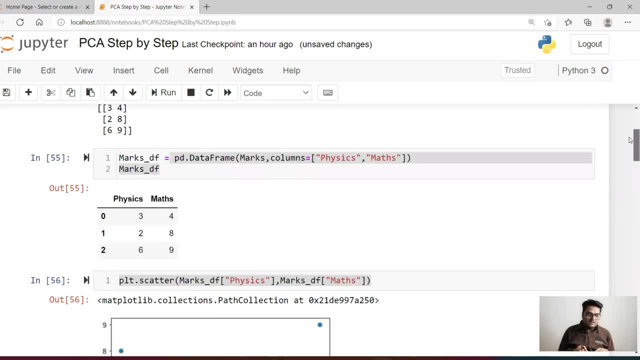 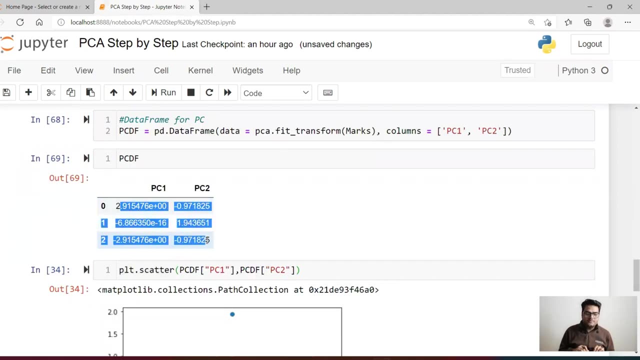 this. So we started from original variables. here, guys, physics, maths- these are the marks. But now physics and maths is not in the picture. Physics and maths are converted to your principal components, and the principal components are looking like this. Now one important concept. 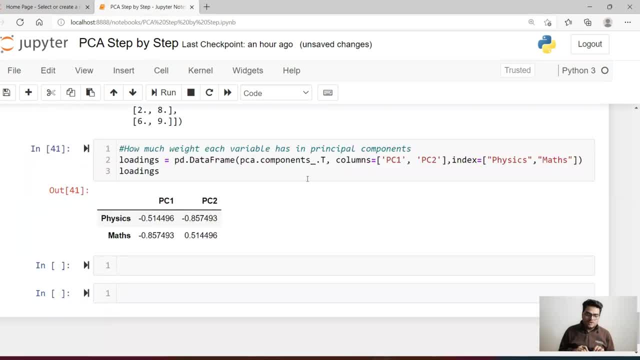 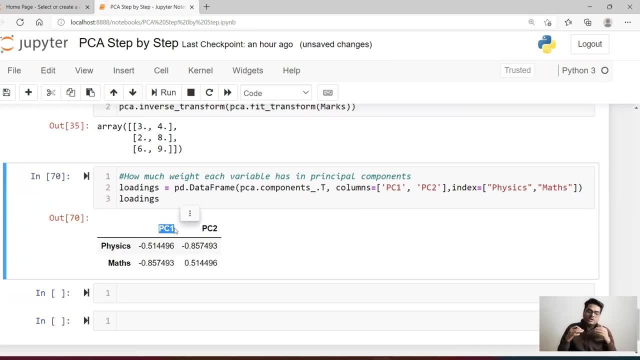 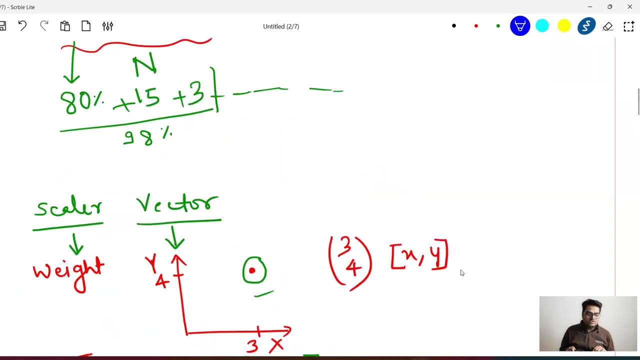 for principal component is loading guys. So I will tell you what is loading. Loading is like how much your each principal components weight from your original variable. So you remember, in the beginning I told you this is a linear combination of your individual variables, principal components. basically, maybe I forgot to tell you in the 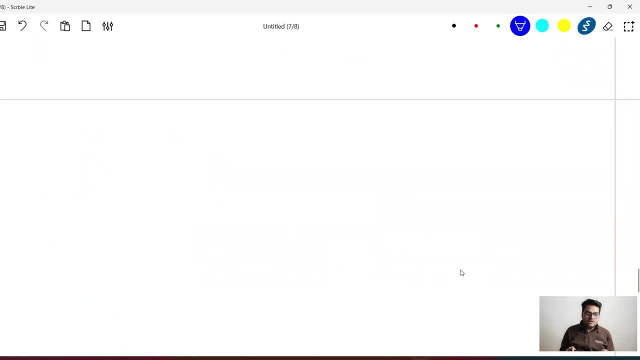 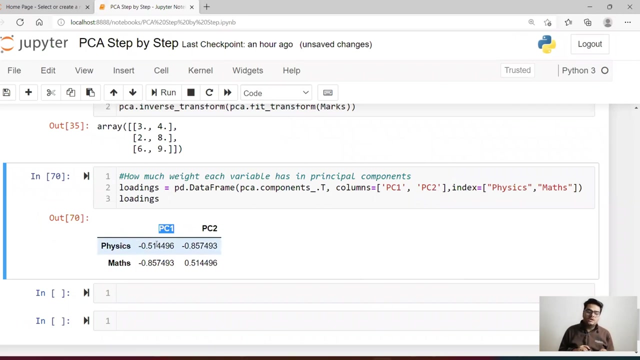 beginning. So PC one. if you ask me, what is principal component one and principal component two? right? So your PC one is alpha one, feature one, plus alpha two, feature two, and so on and so forth. Okay, So what your loading tells you here is physics multiplied by minus 0.51 plus. 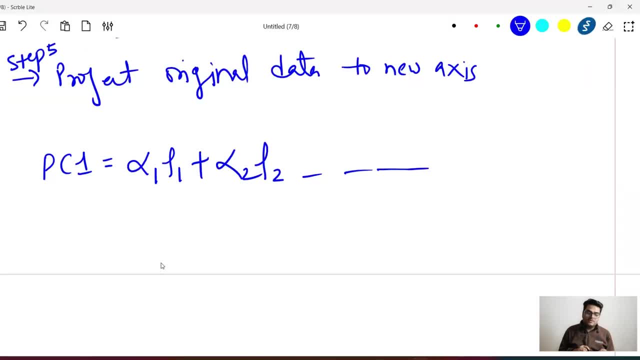 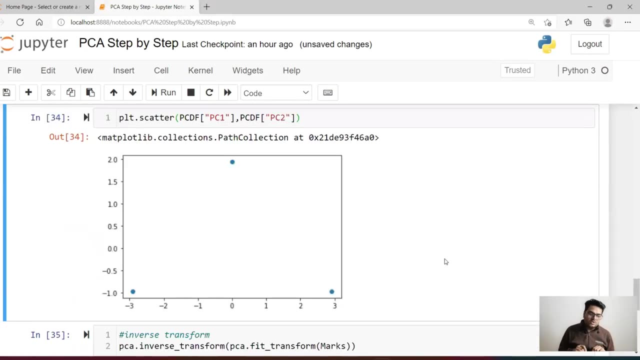 maths, multiplied by minus 0.85 is your PC one. Okay, Similarly for PC two. So your principal components are nothing but linear combination of your original features with some weights. Okay, How can you convert your principal component to original variable? you have to use something known. 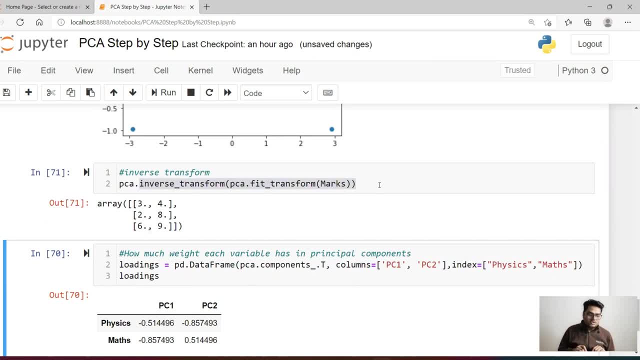 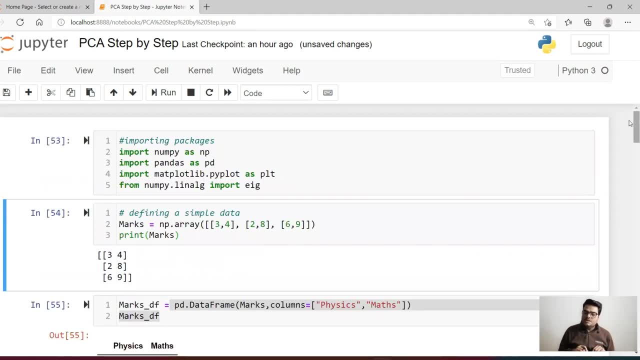 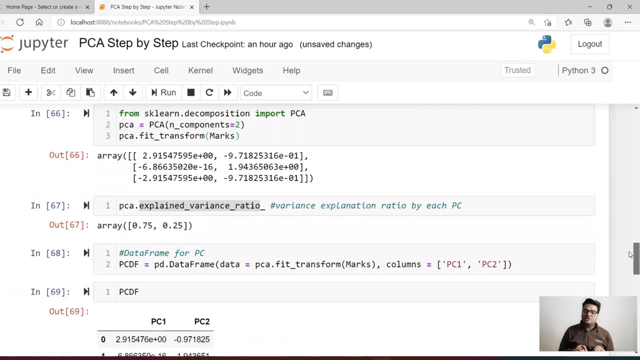 as inverse transform, PC inverse transform. So if you can see, here I'm able to generate the same record that is there in my original data marks. In this case I took a simple data to explain you guys. but if you run it on a bigger data, obviously few initial principal components will be able to explain. 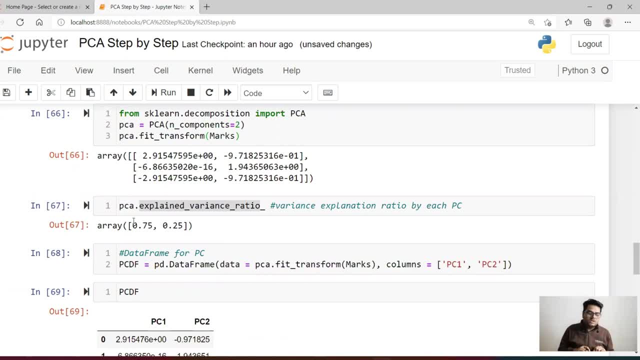 100% of your data variance. Here you can see 100% by these two. if you run on 100 features, maybe first five, six will be able to explain, let's say, 90%. So you take those first five.